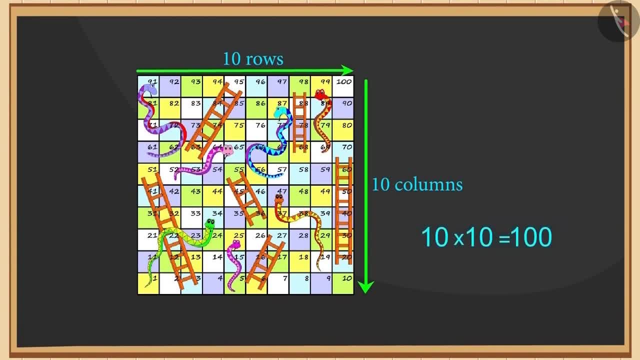 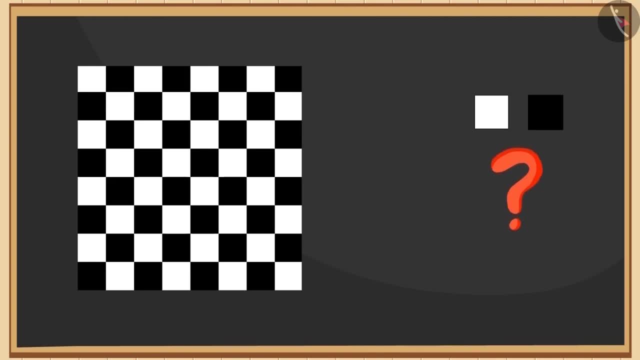 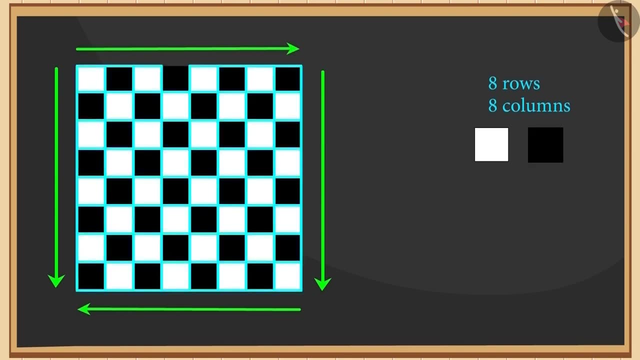 Thus it has a total of 100 small squares. Now look at this chess board. How many black and white squares does it have? Yes, you are right, It has 8 rows of 8 squares each, So it has a total of 64 squares which are either black or white in color, Do you? 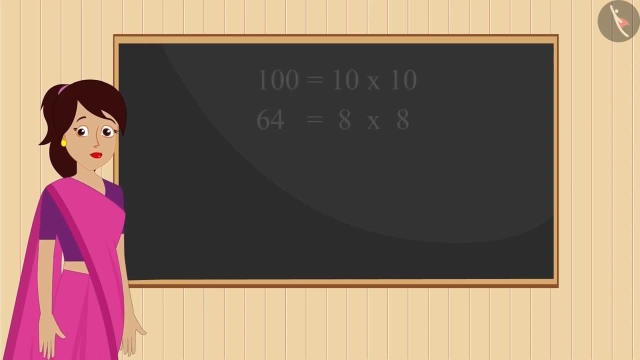 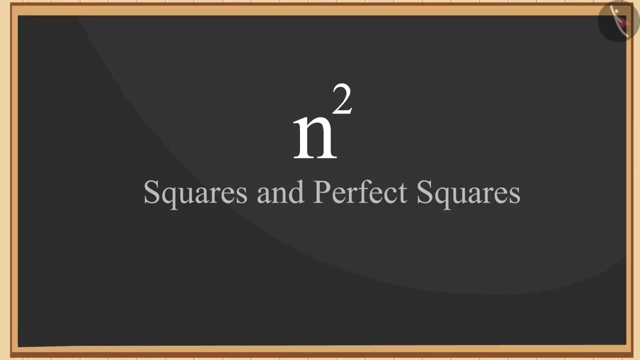 see any similarity between the two numbers. Yes, of course We can write both these numbers as the square of a natural number. Do you know that all such natural numbers which can be expressed as the square of a natural number are called square numbers or perfect? 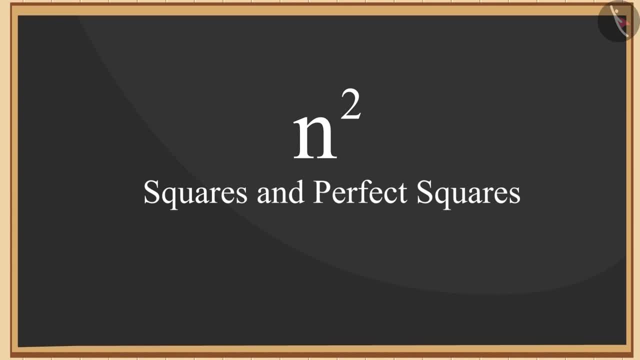 square numbers, For example. look at these numbers. The numbers here are 1,, 4,, 5,, 6,, 7,, 8,, 9,, 10,, 11,, 12,, 13,, 12,, 13,, 14,, 15,, 16,, 17,, 18,, 19,, 20,, 21,, 22,, 23,, 24,, 25,, 26,, 27,, 28,, 29,, 30,, 31,, 31,, 32,, 31,. 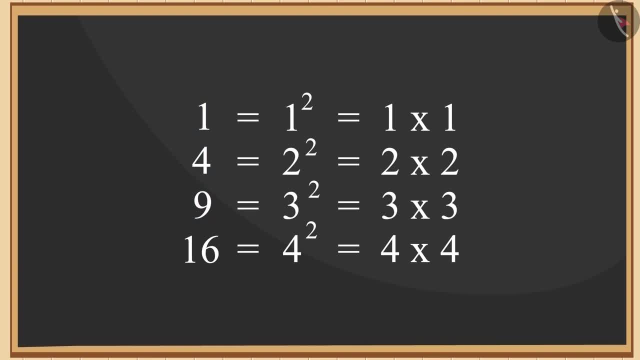 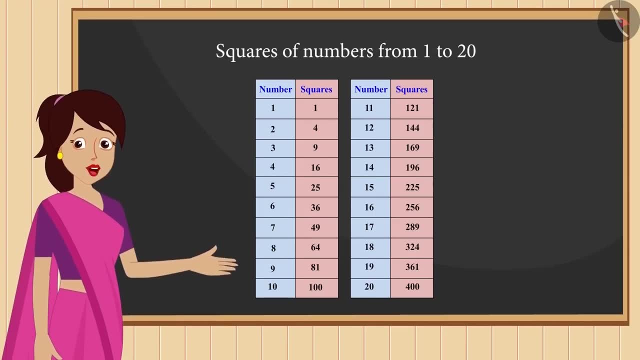 32,, 34,, 35,, 36,, 37,, 38,, 39, 40.. The numbers here, 1,, 4,, 9 and 16 are square numbers. Let us now look at the squares of numbers from 1 to 20.. If you wish, you can pause the. 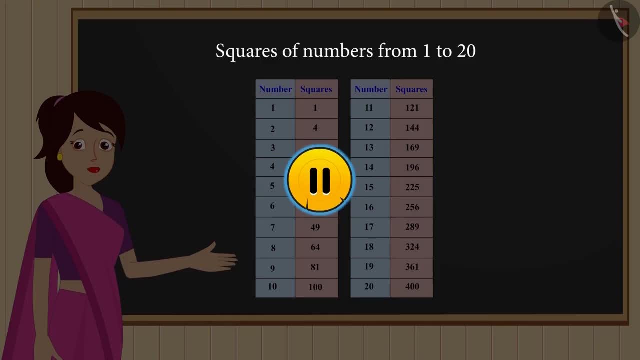 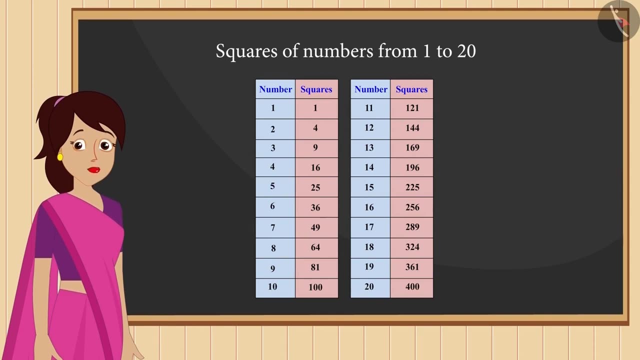 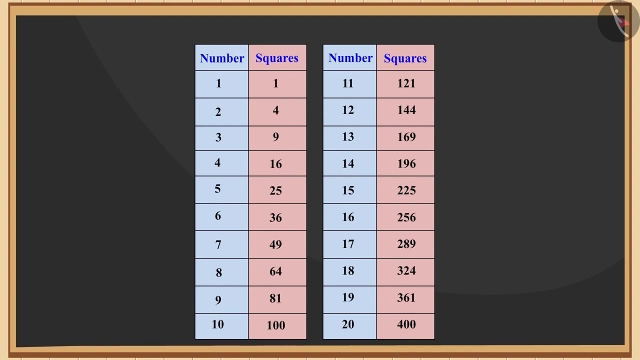 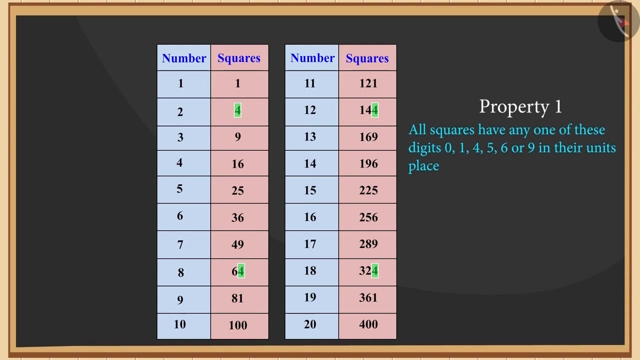 video here and write the squares in your notebook. After writing the squares of the numbers from 1 to 20, you must have got this type of a table of squares. Notice the digits in the units, please, of these squares. Yes, you will see that the squares have any one of these digits: 0,, 1,. 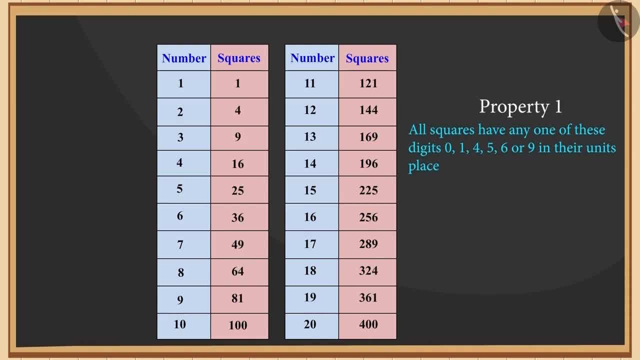 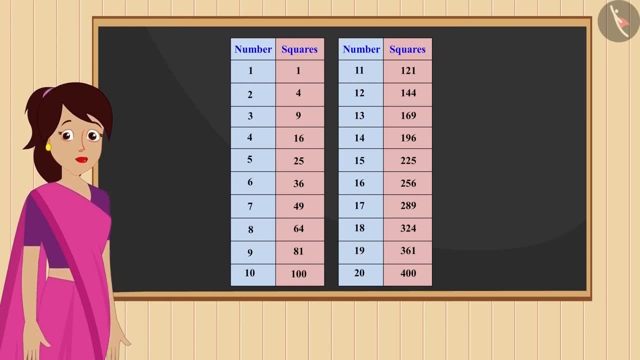 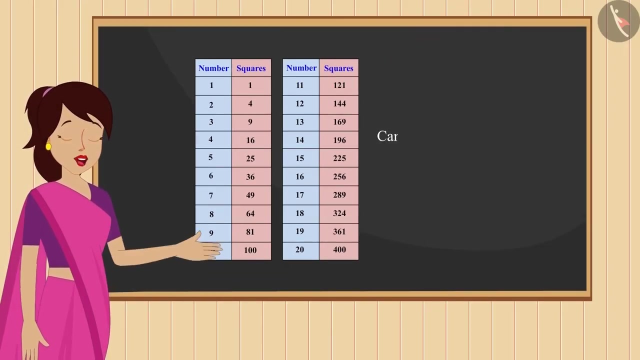 4,, 5,, 6 or 9 in their units place. Now you may wonder whether this is valid for all perfect squares. Yes, it is valid for all perfect squares. If you wish, you can pause the video here and check other squares as well. But can we say that every number ending with 0,. 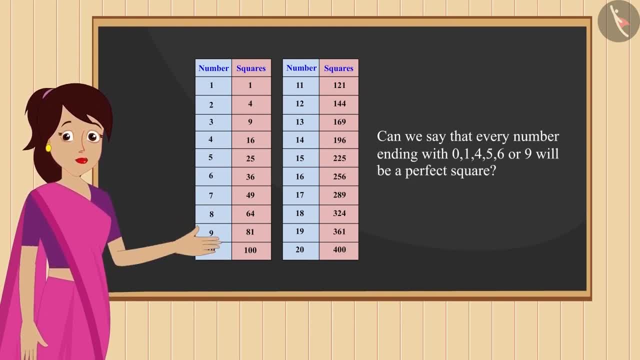 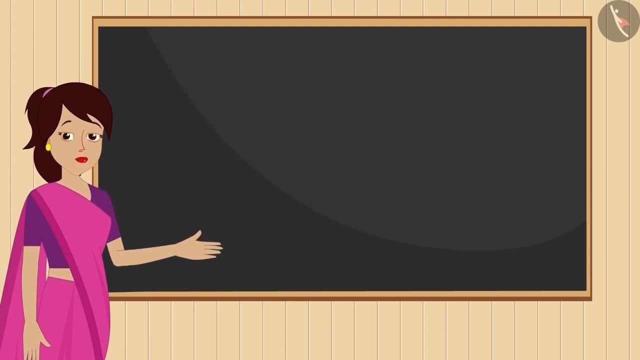 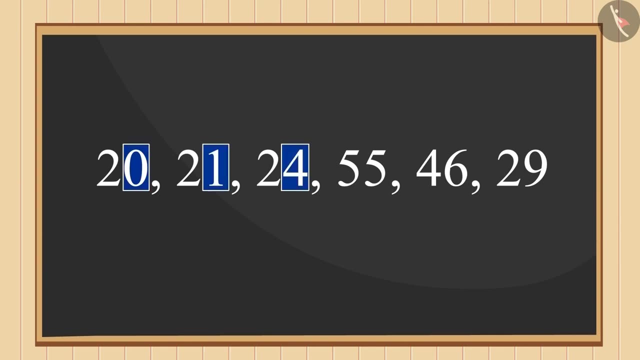 1,, 4,, 5 or 9 will be a perfect square. Come on, let's examine some such numbers. Take a look at these numbers. All of them have either 0,, 1,, 4,, 5, 6 or 9 in their units place.